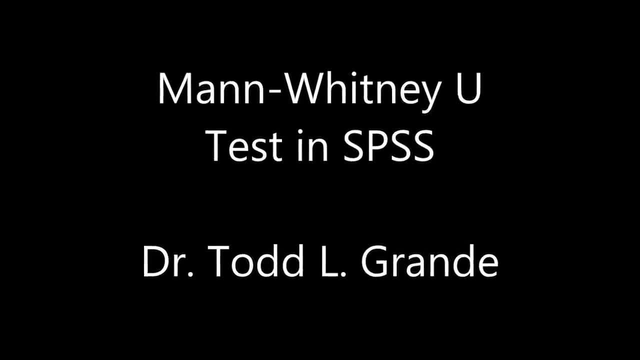 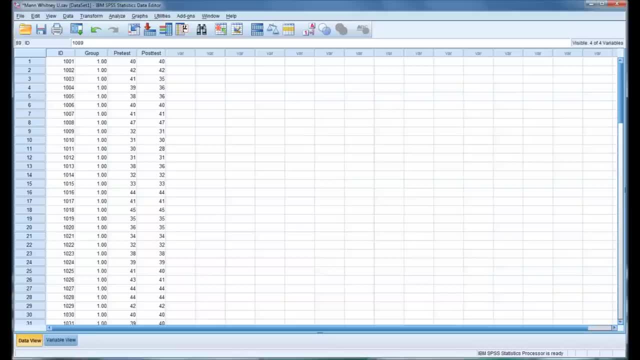 Hello, this is Dr Grande. Welcome to my video on how to perform a Mann-Whitney U-Test using SPSS. The Mann-Whitney U-Test is a non-parametric test. A lot of the statistics we use in counseling. 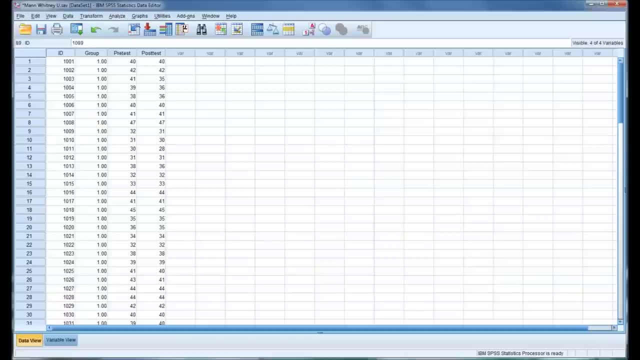 research are parametric tests. For example, the ANOVA is a parametric test And it requires continuous or scale data, For example, interval or ratio data. A non-parametric test allows you to perform similar calculations using ordinal data Or a mixture of ordinal and continuous data. So I have here an SPSS data set with some fictitious 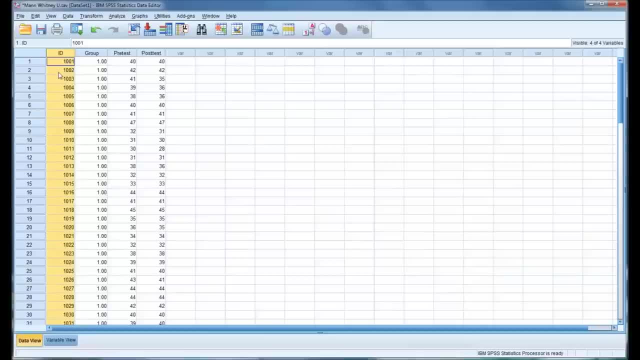 data. You can see in the first variable's ID and there's 90 participants in this study And you can see the next variable's group. You have a control group of 45 of the participants and a cognitive behavioral therapist And you have a control group of 45 of the participants and a cognitive behavioral 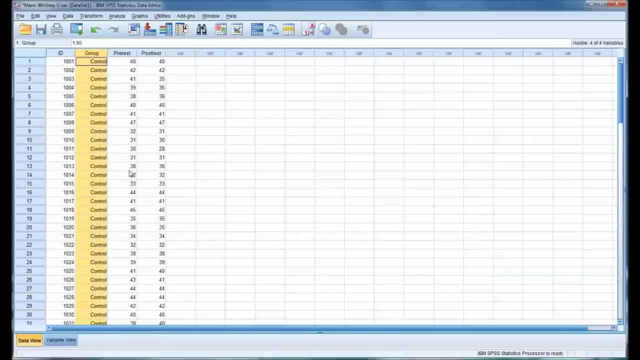 therapist And you have a control group of 45 of the participants and a cognitive behavioral therapist, And you have a control group of 45 of the participants and a cognitive behavioral therapy group for the other 45. And then you have a pre-test score and a post-test score. So let's 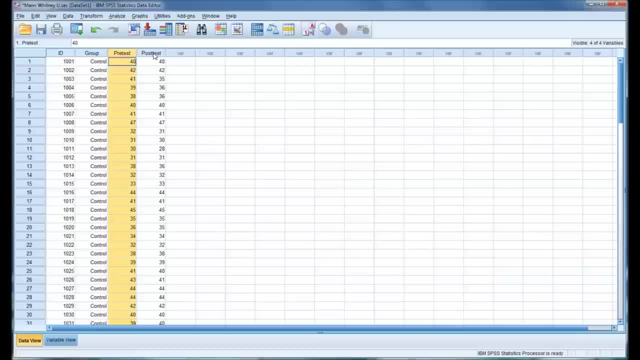 assume that this instrument is the same. The pre-test and post-test instrument is the same. The scores come from the same instrument And it measures depression, And a low score represents less severe symptoms of depression And a high score represents more severe symptoms of depression. 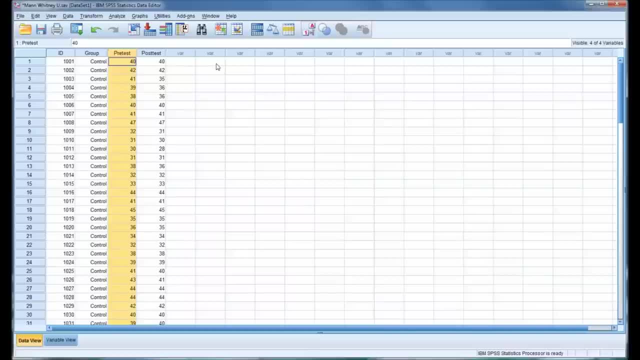 And let's assume we want to test if there's a difference between the control group and the CBT group on the pre-test and on the post-test using the Mann-Whitney U-test. So go to Analyze and then to Nonparametric. 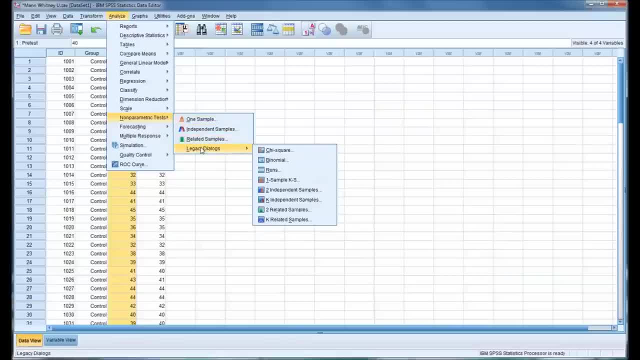 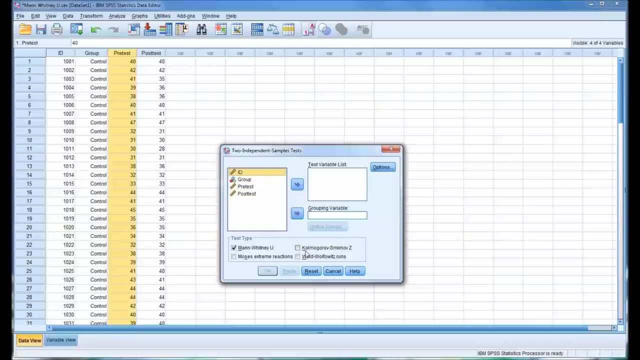 Tests And there are a few ways to run nonparametrics in SPSS. I'm going to show you this way first. So this would be a way to run the Mann-Whitney U. You can see down here it's checked off Mann-Whitney U And for the test variable list. 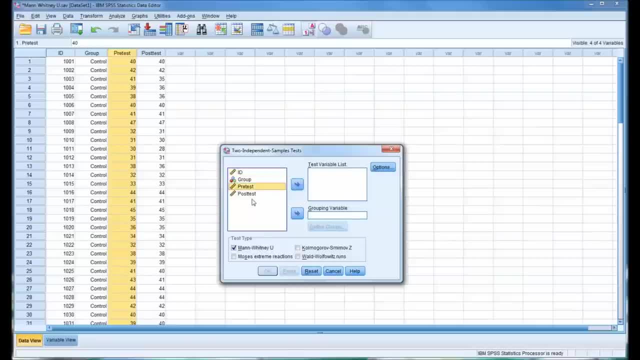 this is the same as the dependence right. So that would be pre-test and post-test And of course your grouping variable will be group, And then you can see it has these question marks here in the parentheses And it's asking you to define the groups. Now I've defined the control group as: 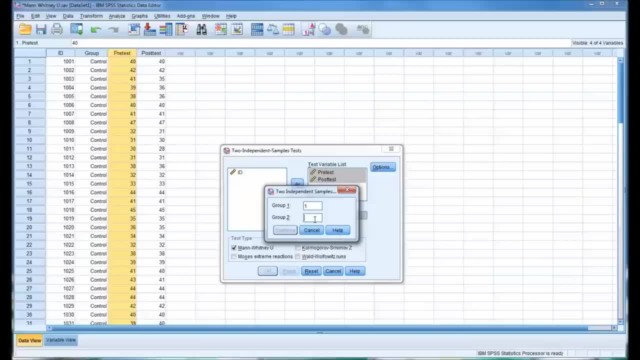 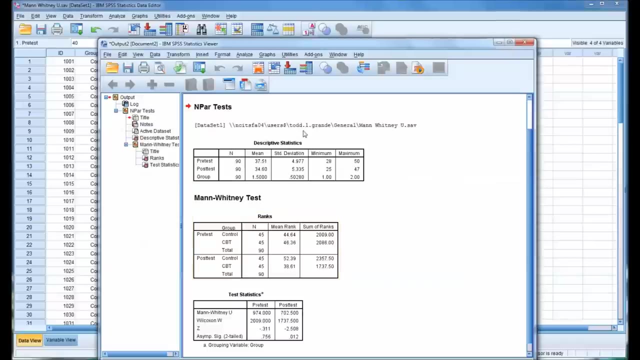 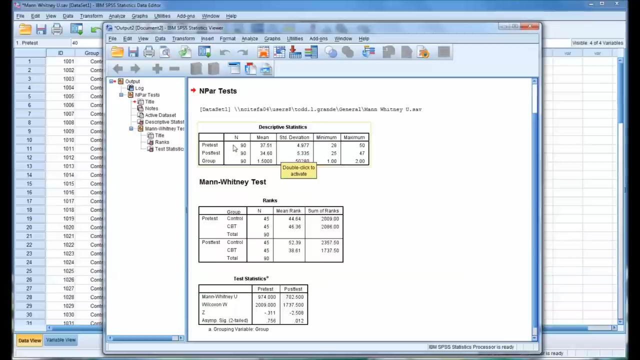 value of 1. And the CBT group as value of 2.. And, of course, in Options you have a few options. We'll have the descriptive statistics displayed And click OK And you can see the descriptive values. to start with, We have the 90 participants in the pre-test and post-test. It gives you the mean, the standard deviation and the 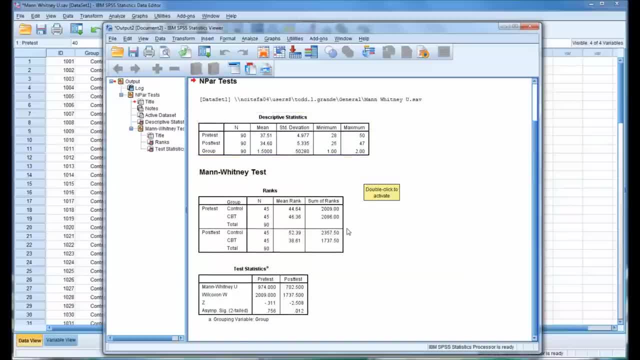 minimum and maximum values. And then you can see the ranks here for the control and CBT for the pre-test and the control and CBT for the post-test And you can see there's a little difference here and a greater difference down here with the post-test. And then you can see the. 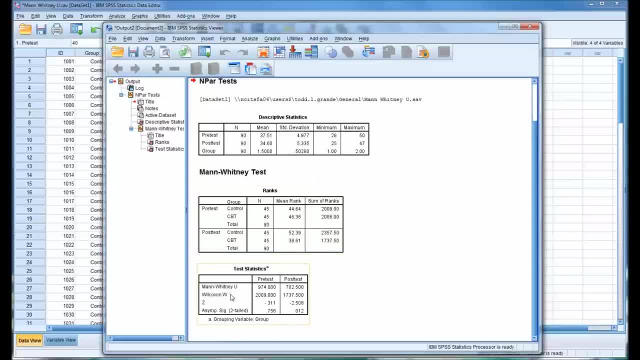 number 0 and 0 for the pre-test And then for the test statistic itself you have the Mann-Whitney U And we're interested in the significance down here. so for the pre-testThere was no statistically significant difference between the control group and the CBT group, But for the post-testthere 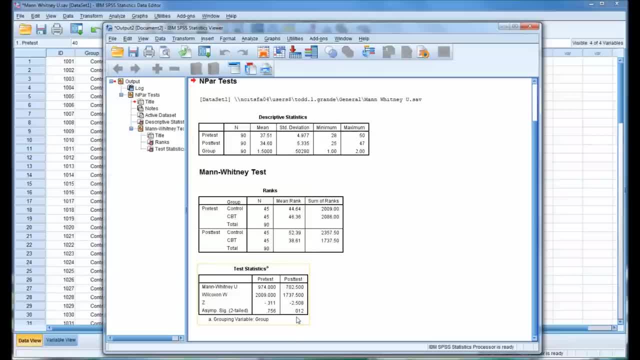 There was .012. That's. that represents a statistically significant difference between the control group and the CBT group. in a簡單 personas, In regard to the Mann-Whitney u-test compared to the Kruskal-Wallis test, I want to show: 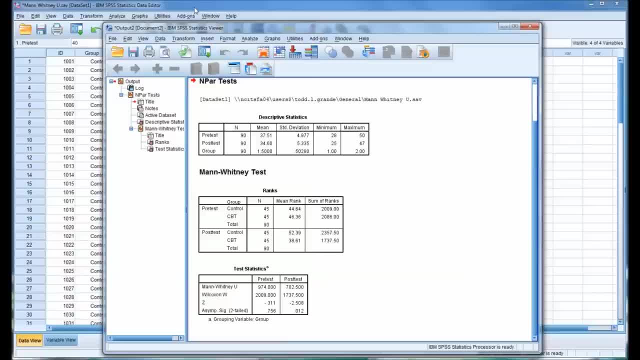 you something interesting: The Kruskal-Wallis test is the nonparametric equivalent of one-way ANOVA. Now you remember these values- 0.756 and 0.012, so I'm going to go back to Analyze. 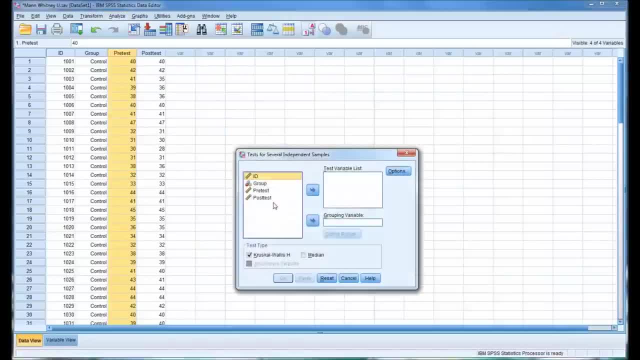 and Nonparametric and I'm going to run a Kruskal-Wallis h-test And I'm going to set the variables up in the same way and define the grouping variable in the same manner. So I set up exactly the same, except the Kruskal-Wallis h-test instead of the Mann-Whitney u. 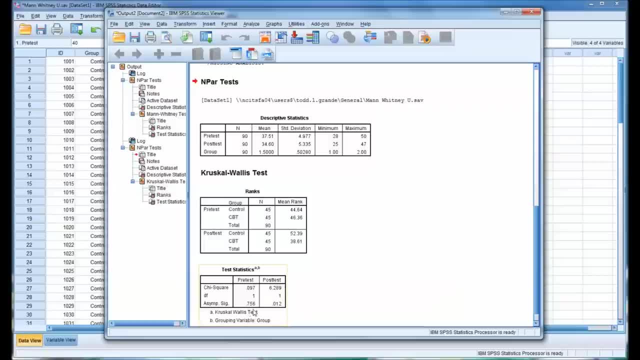 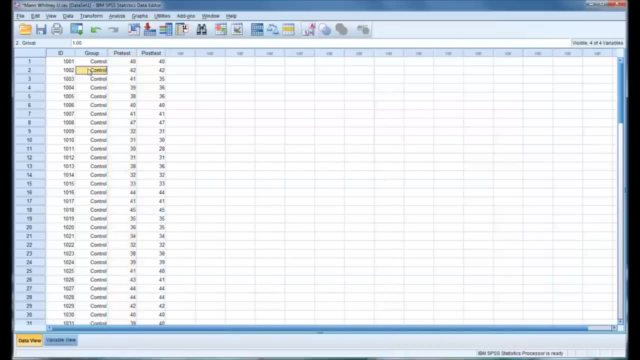 OK, And you can see that the significance values are identical. The difference with the Kruskal-Wallis test is that it can handle more than two levels of the independent variable. So if I go back here to the data set, you can see I have control and then the CBT. 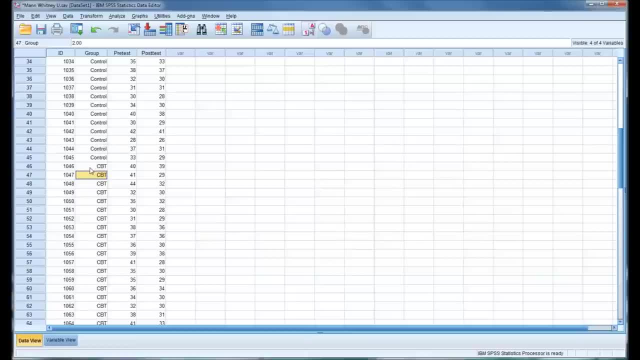 and you have 45 participants in each group, But say that you had 30 participants in control and then 30 in CBT and then say down here 30 in existential therapy, for example. The Kruskal-Wallis H test could analyze that data. 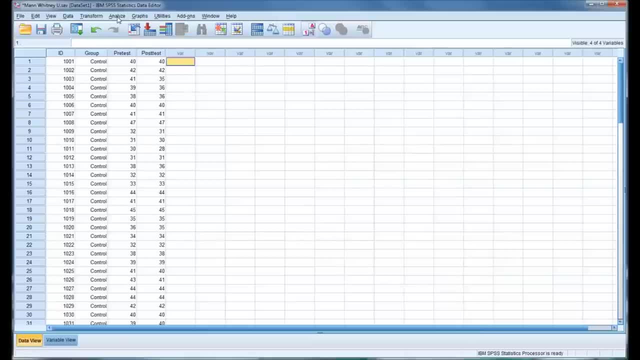 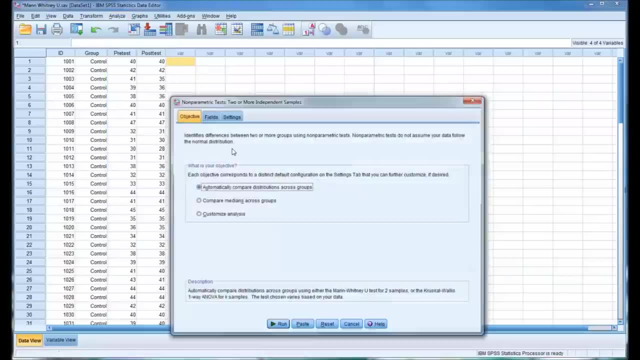 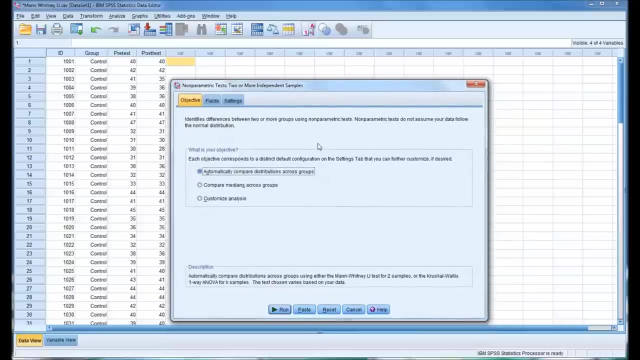 So now I'm going to show you another method to run the Mann-Whitney U test. If you click Analyze and go to Non-Parametric Tests and select Independent Samples, you're going to see this dialog appear that does not look the same as the dialogs typically appear in SPSS. 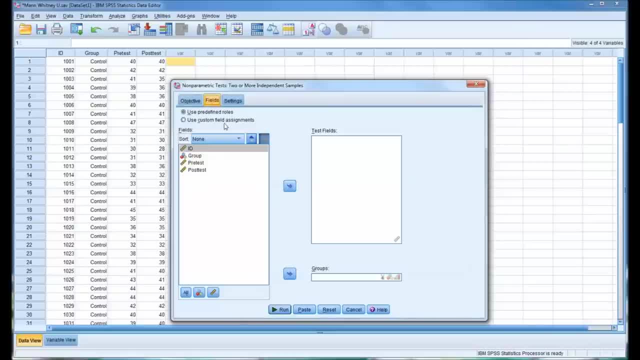 This Objective tab. skip this and go to Fields And the Test fields. you want to move over the Pre-Test and Post-Test And the Group. you want to move that to Groups, the Groups field, And then move to Settings and see the default. 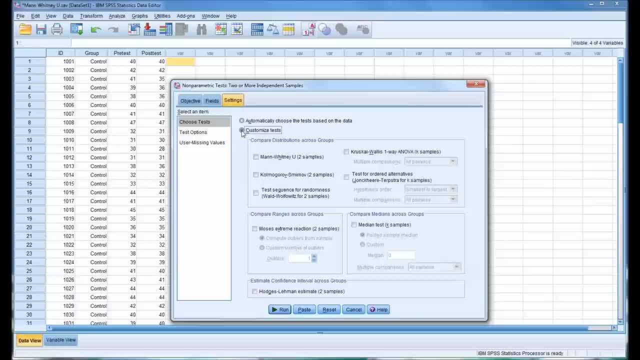 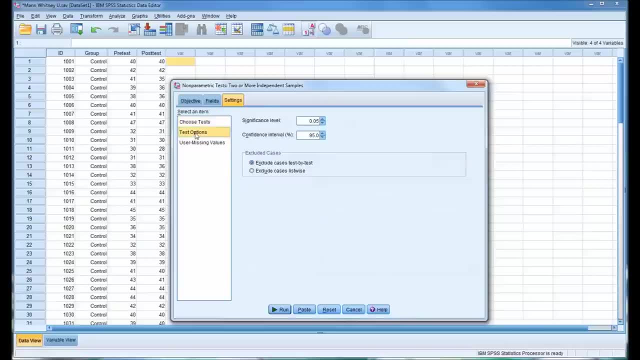 You can see it's automatically choose the test. but go ahead and click Customize Test and select the Mann-Whitney U And then you can click Test Options. You can see the significance level is set by default at 5% And we'll leave the missing values set at Exclude by default. 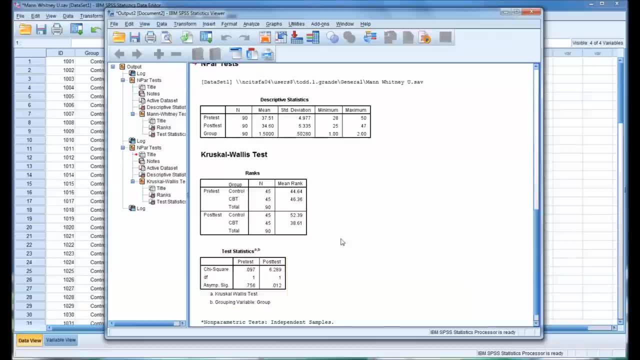 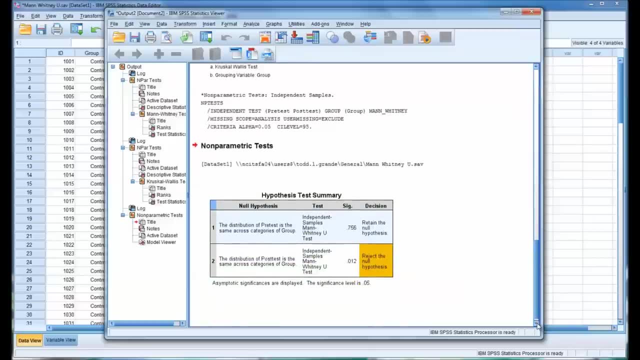 And then you'll click Run down here And you can see the output is also not the same as we're used to seeing in SPSS. So you have the it states, the null hypothesis. the distribution of Pre-Test is the same across the categories of Group. 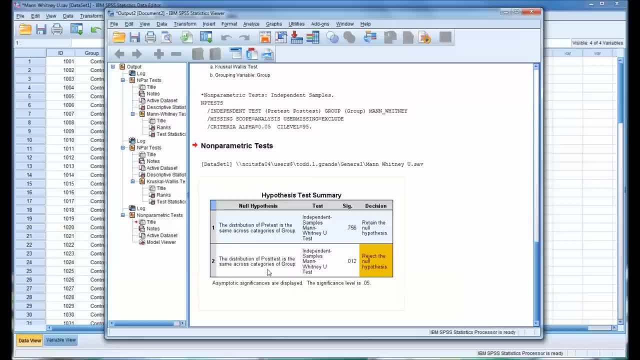 And of course, the null hypothesis down here is: the distribution of Post-Test is the same across the categories of Group And you can see the same values appear. It's just the way it's displayed is not the same If you double-click this. 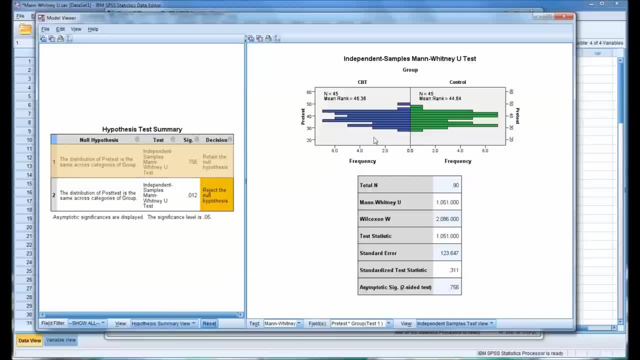 So you can see here the frequency for CBT and for the Control Group. Now note: this is for the Control Group. I have it selected over here. If I selected the CBT group, it would switch, so let's stay with the control group. we can see the. 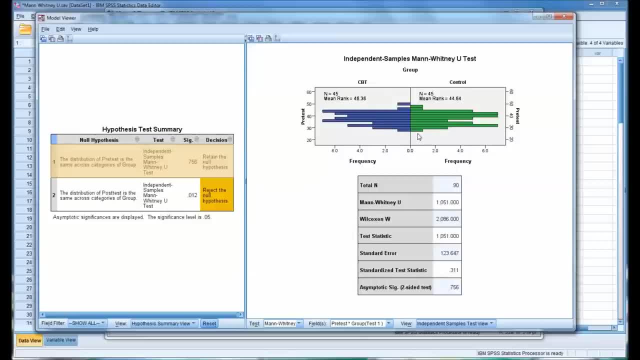 frequencies are fairly similar, so this makes sense that the null hypothesis would be retained and you can see the value of the bandwidth you test statistic, which you'll need for reporting, and, of course, the significance level, and there's a few other options that you may want to use. you can see. 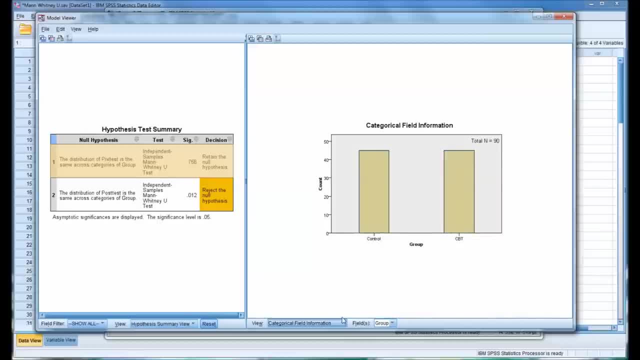 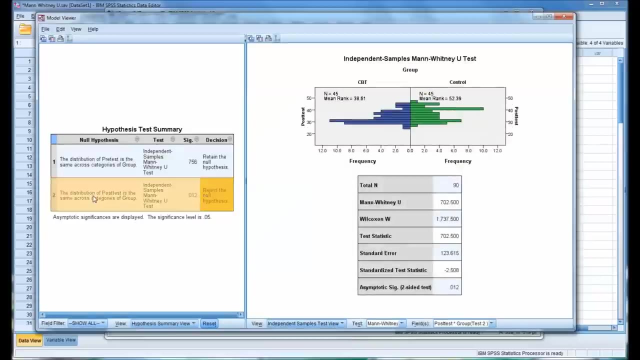 categorical field information, which, of course, you already know- the sample size and the group size, and then continuous field information is available as well. so if we move to the CBT group, we're going to reject the null hypothesis because the significant level, the significance level, is below 0.05, and you 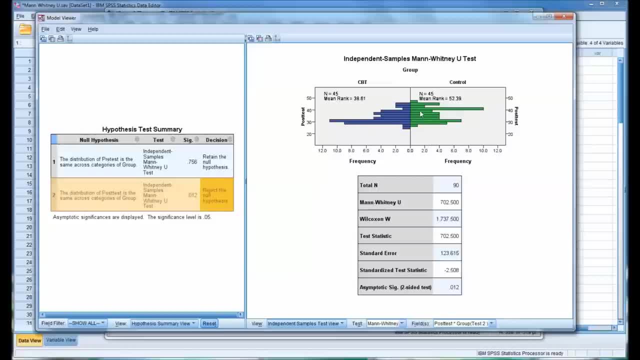 look at this frequency, you can see that it is quite different. so that would make sense that the two groups are. you can see that it is quite different, so that would make sense that the two groups are. so that would make sense that the two groups are statistically significantly different. again, here's the test: statistic and the 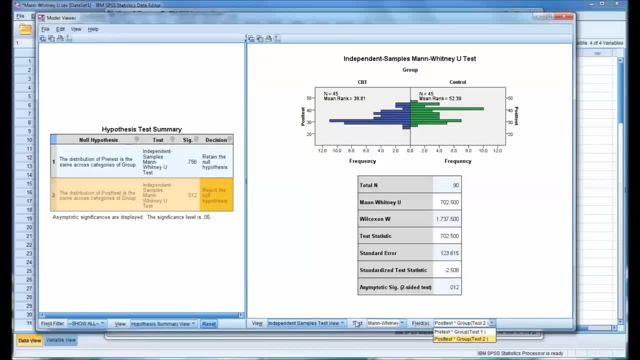 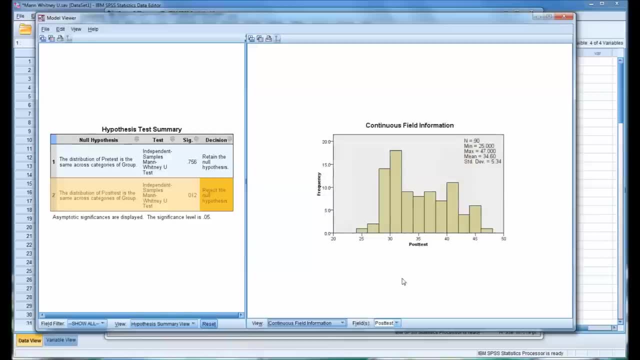 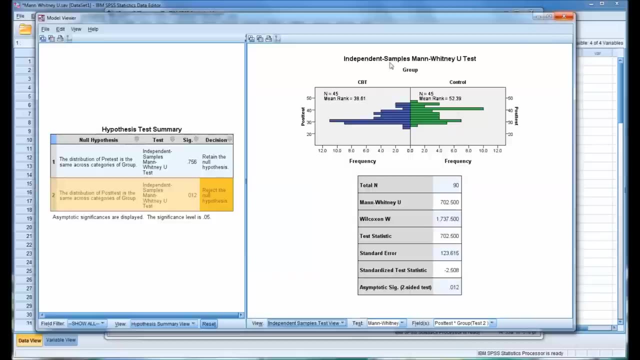 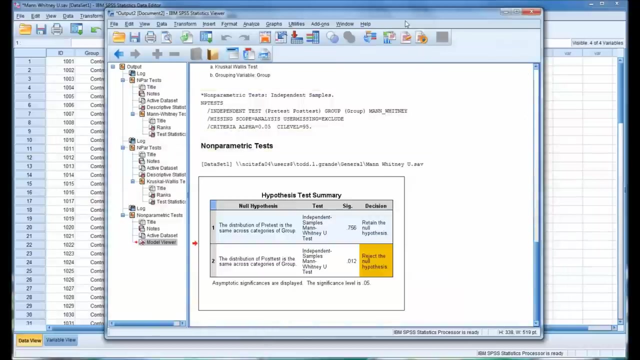 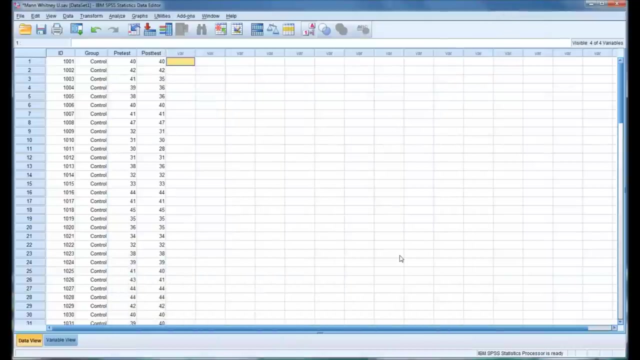 significance and similarly over here you can look at the categorical field information and the continuous field information. so that's just a different way of running the same statistic and the outputs much different and the dialog box is also different. I hope you found this video on the Mann Whitney you test.